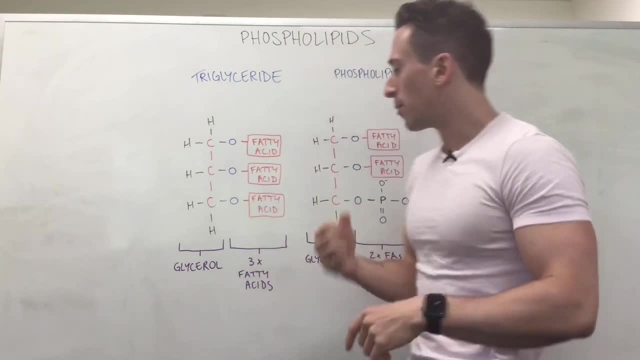 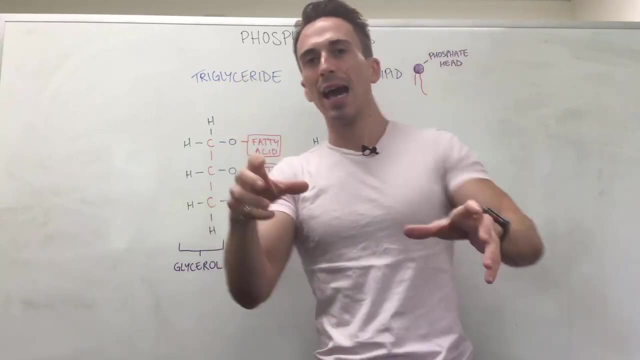 is the way that our body stores fats and it's made up of a glycerol backbone. That's the glycerol here, Three carbons- You can see the hydrogens- and three oxygens, and it's attached to three individual fatty acids. And I told you it can be many different types of fatty acids. They can be: 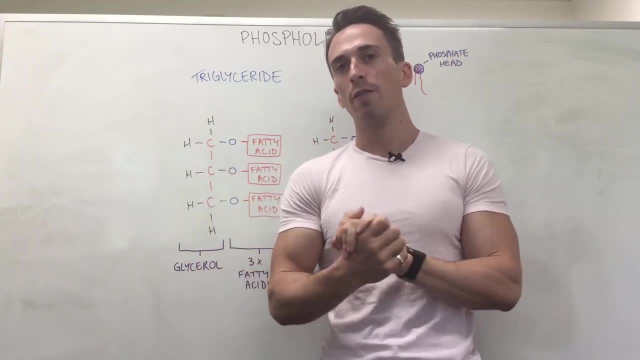 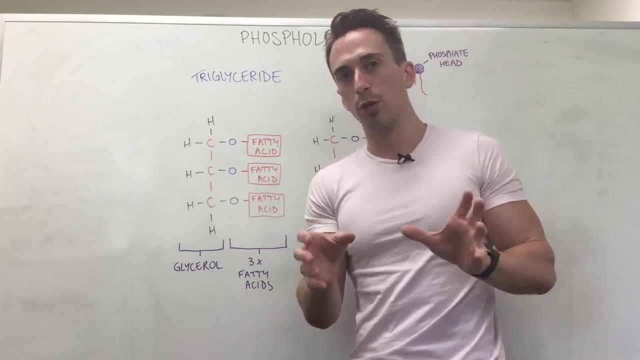 saturated, monounsaturated or polyunsaturated And, depending on the quantity of each of those, depends on whether it's going to be a liquid or solid at room temperature. So this is a triglyceride. It doesn't like water because there's not many. 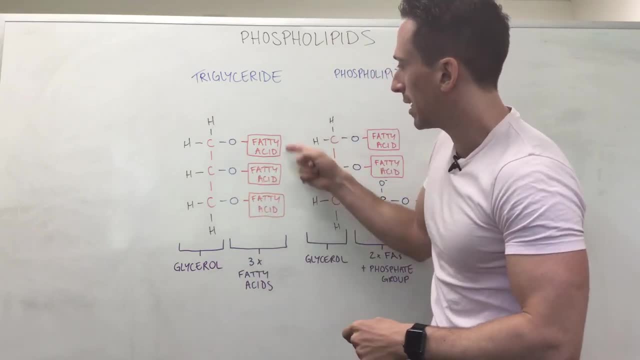 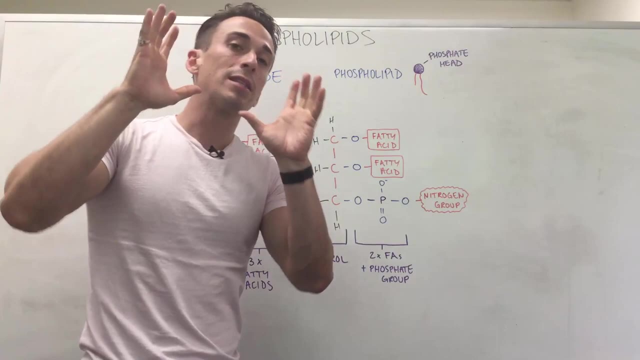 oxygen molecules. There's a huge amount of carbons and hydrogens here, with the fatty acids, Big long hydrocarbon chains. Now let's compare this to a phospholipid. Now let's look at the similarities. first, There's a glycerol backbone, That's the same. So you can see the three carbons, the 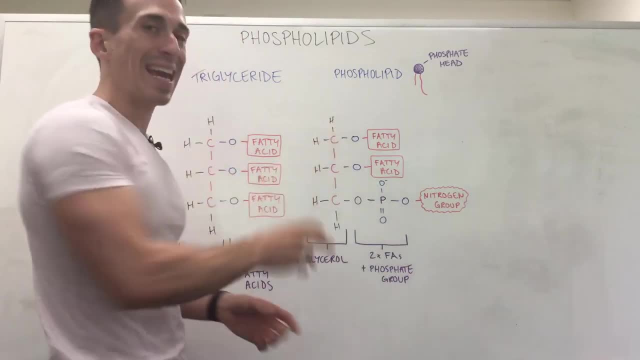 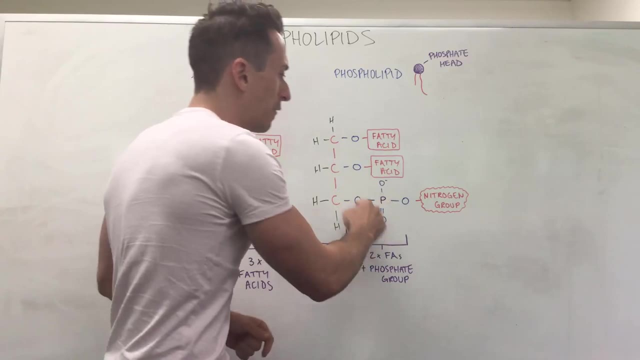 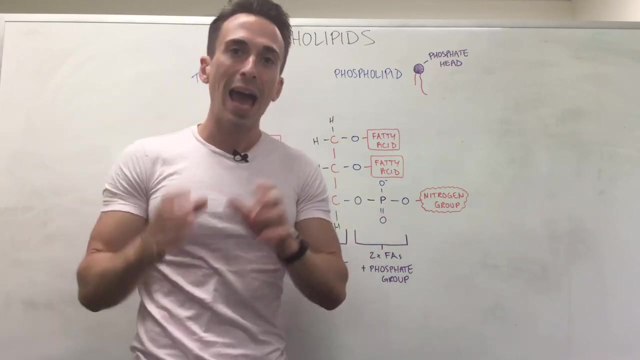 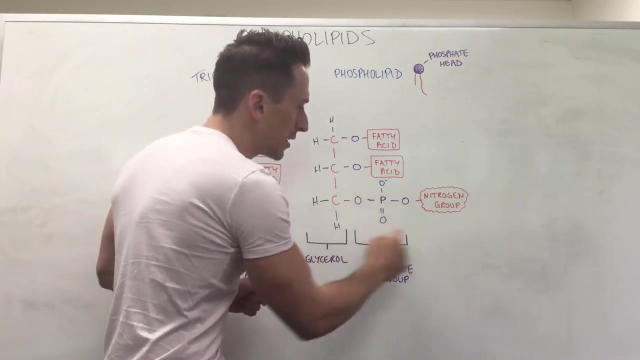 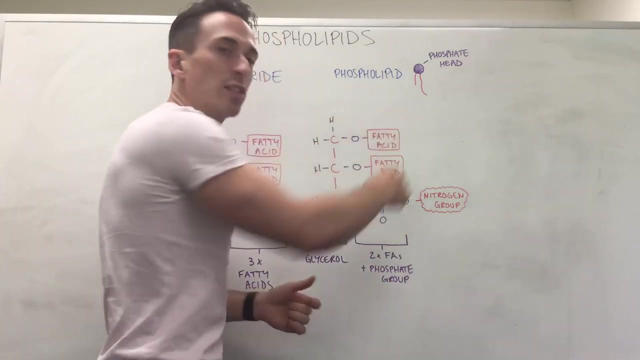 hydrogens and the oxygens, And it's similar to a phospholipid. Now let's compare this to a glycerol backbone. It's still got two fatty acids attached to it, But in the position where the third fatty acid would attach in the triglyceride, what we have is a phosphate group attached in, And you can see that this phosphate group has a large amount of oxygens attached to it as well, And attached to that is a nitrogen group as well. Now, what this means is that, because of this additional phosphate group, one part of this molecule loves water and the other part of this molecule hates water, And it 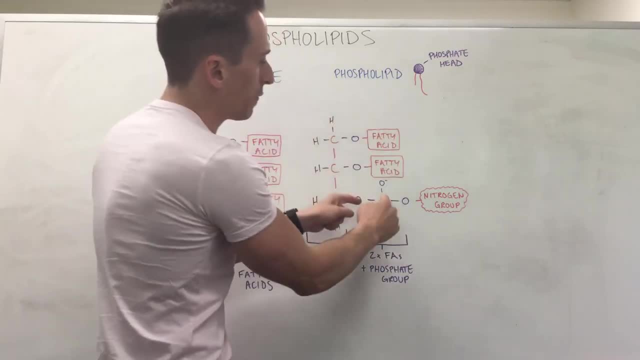 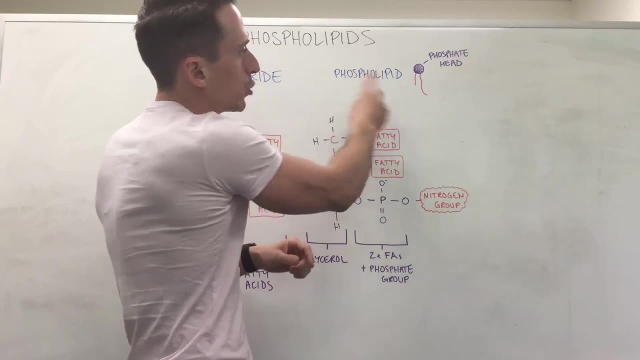 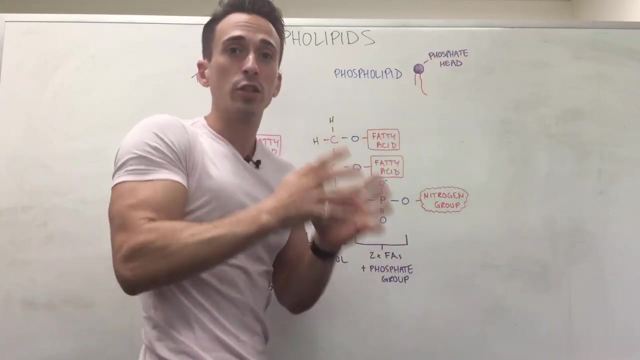 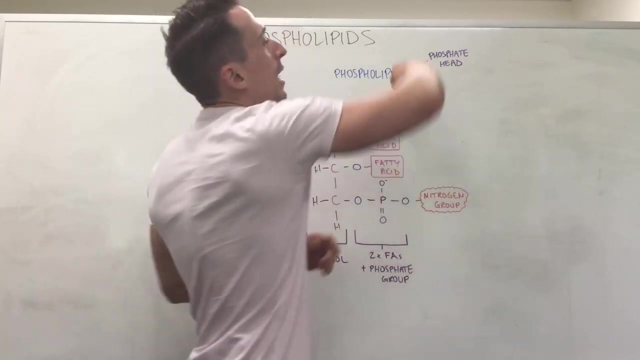 actually arranges itself in a way that looks like this, where the phosphate pops itself away from the rest and creates a phosphate head, And then those two fatty acids form two fatty acid tails, And that means that we have a part of a phospholipid that loves water- that's the phosphate head- and a part of a phospholipid that hates water- that's the fatty acid tails. Now, what that also means is, when we've got heaps of these phospholipids, they will spontaneously arrange themselves in a way in which